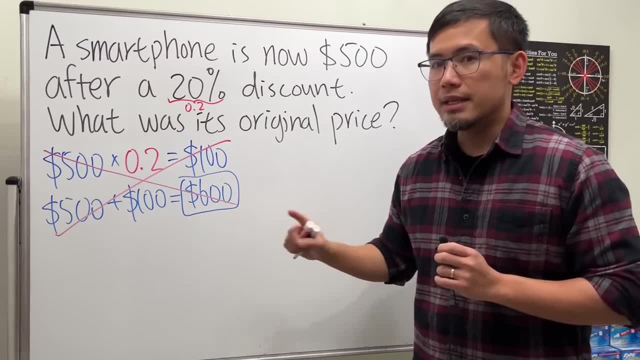 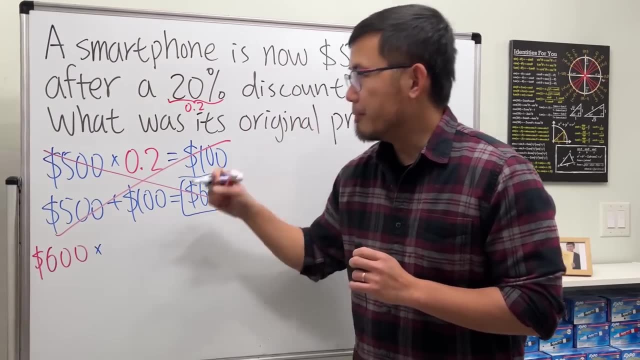 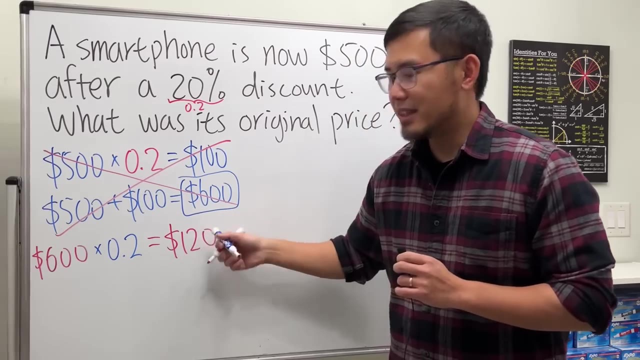 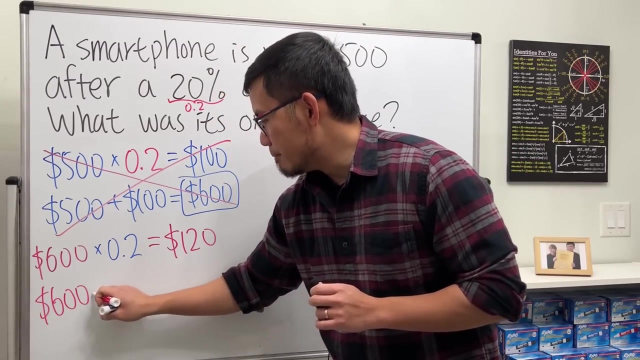 if you take 600 dollars as the original price, and let me just write this down- and if you multiply this by 20%, which is again 0.2,, you will end up $120. And then if you start with the original $600 and then minus the $120,, 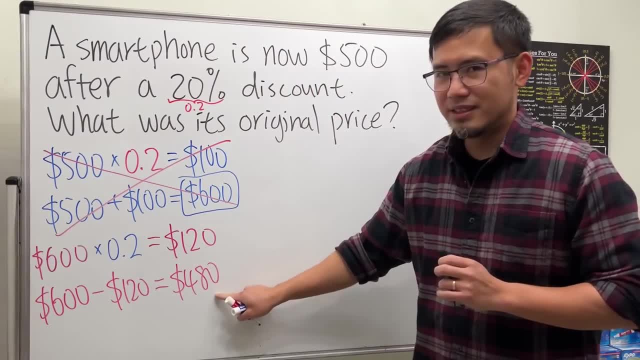 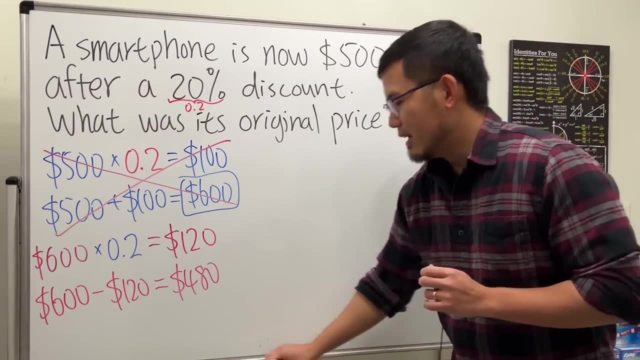 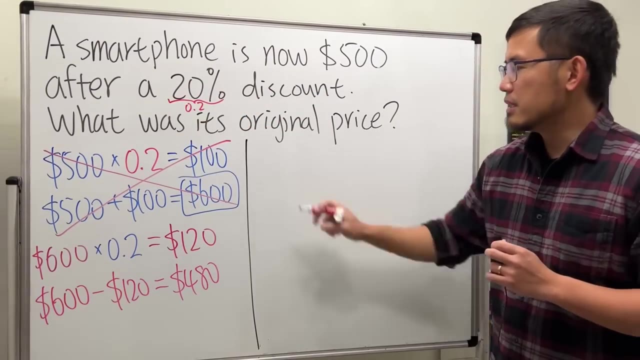 you will end up $480.. So this is not the same as the $500 that we are looking for. So this is not correct. So how exactly do we do it Here? let me show you guys a fast way. The key is the 20% discount. 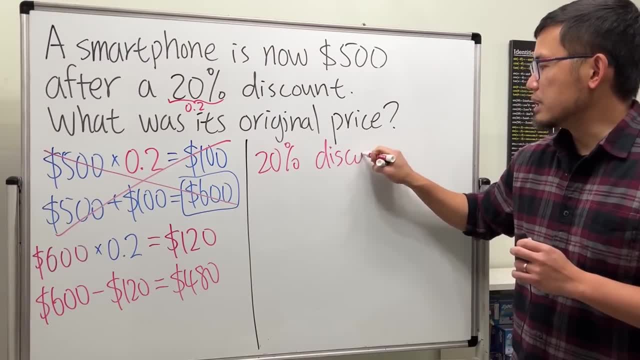 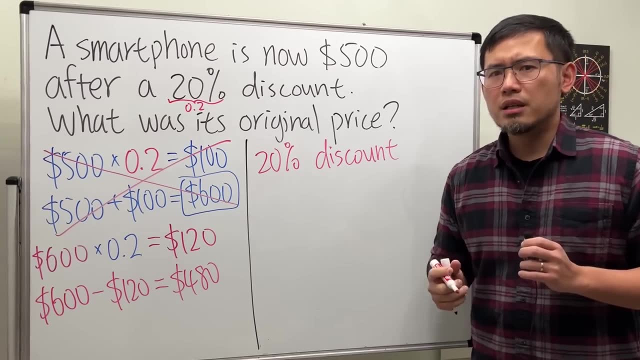 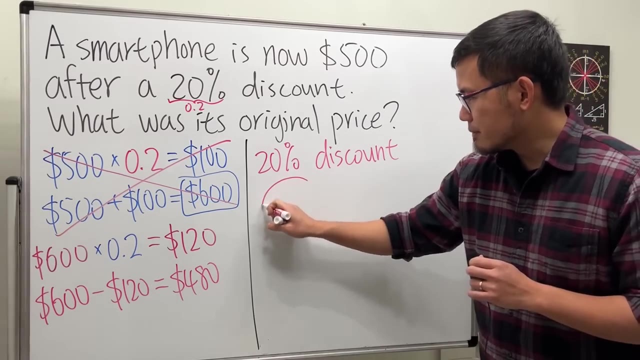 So now let's think about it. What exactly does the 20% discount do for us? Well, originally we will have to pay for the full price, right? And what percentage is the full amount? Let me draw a picture for you guys, right here, Let's say this right here, is 100%. 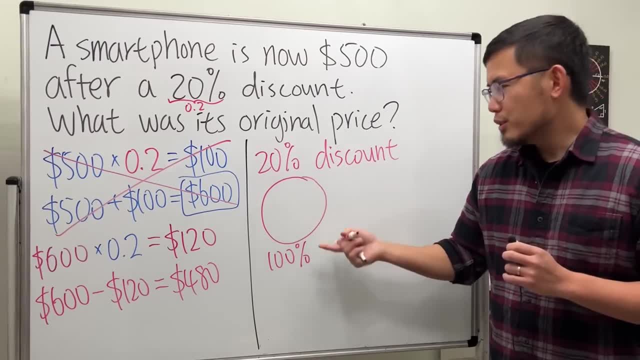 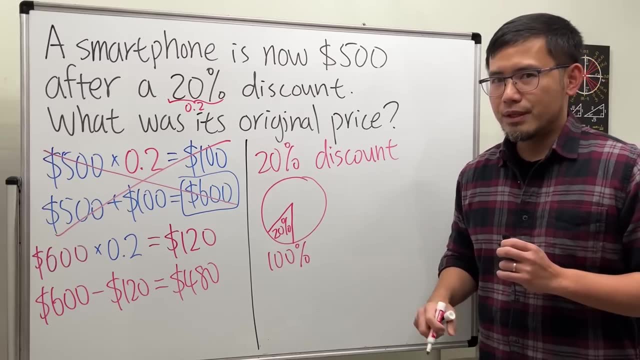 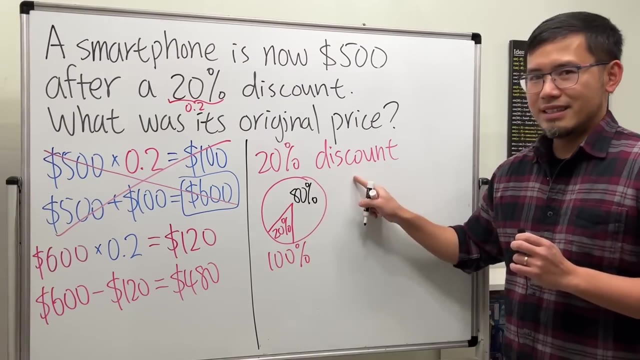 But now we have a 20% discount So you can just think about it like: okay, you don't have to pay that 20% right here anymore. So what percent do we have to pay? The remaining is what? 80% Right, Because together we have to get 100%. 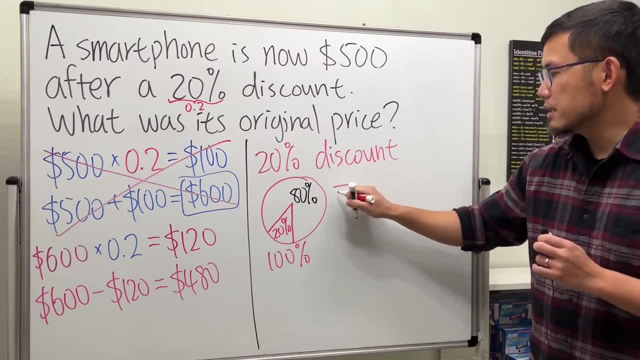 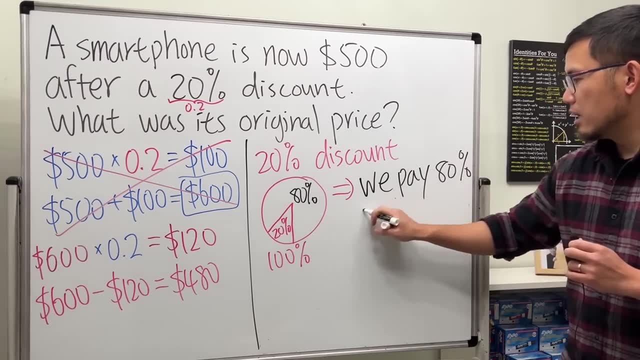 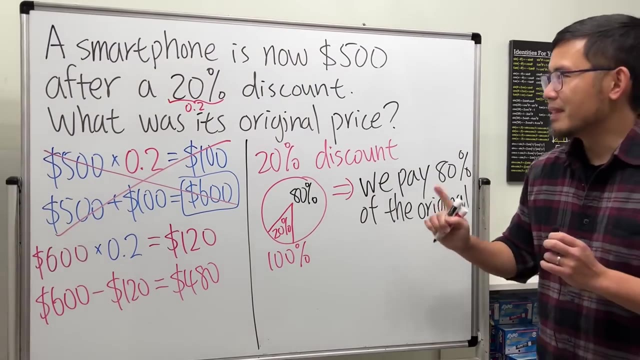 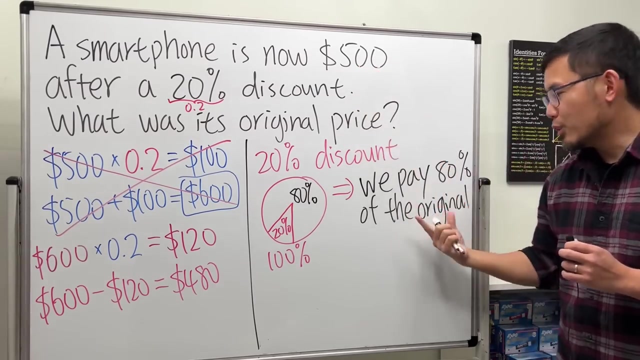 so, when we have a 20% discount, this means we pay 80% of the original. and now let's think about it: 80% of the original, which is the sell price, which is 500. so how can we figure out the original? well, 80% of means we multiply 80% times the. 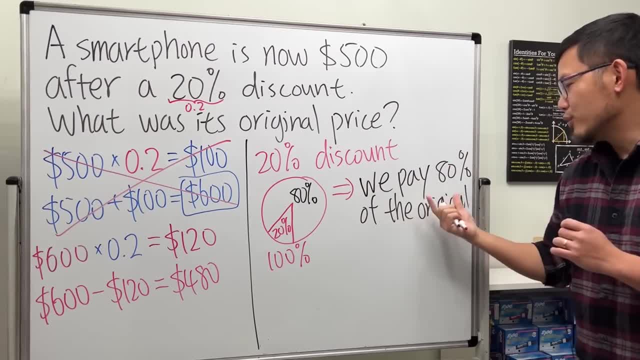 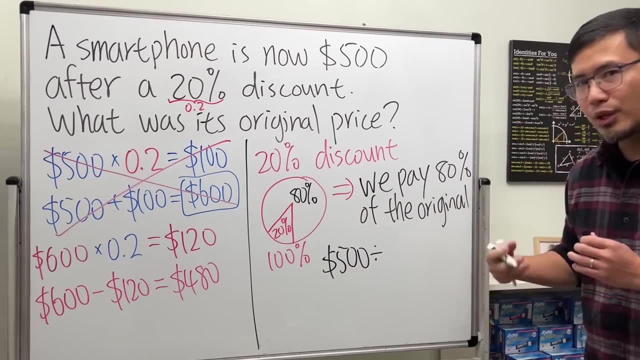 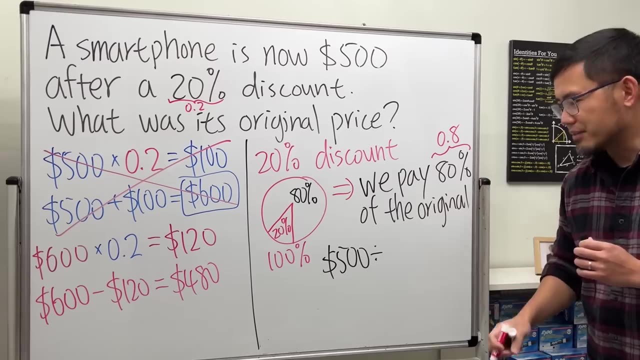 original gives us 500. so if I want to figure out the original, just go ahead and do $500 right here. divide, because we have to do backwards. divided by 80%, which is 0.8, by moving the decimal twice to the left. all right, okay, just real. 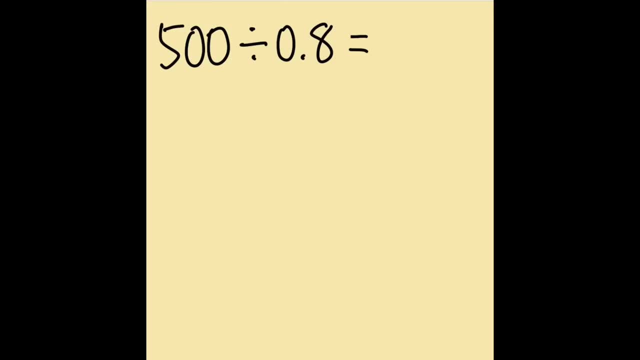 quick: 500 divided by 0.8. let's use long division and remember the first number goes inside and the second number goes on the outside. so that's the setup. but for the outside number we don't want to have a decimal. so change that, we just have to move the decimal point.